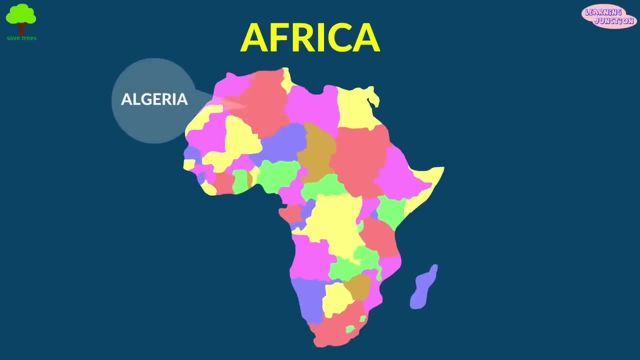 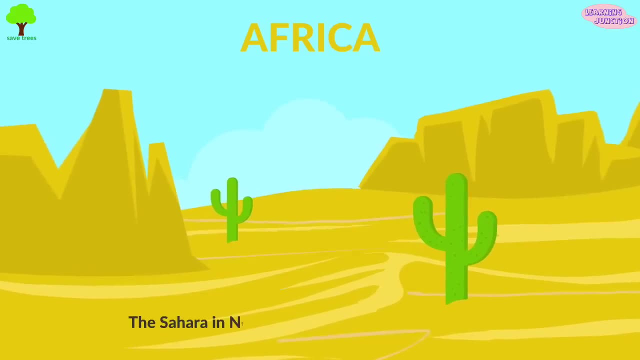 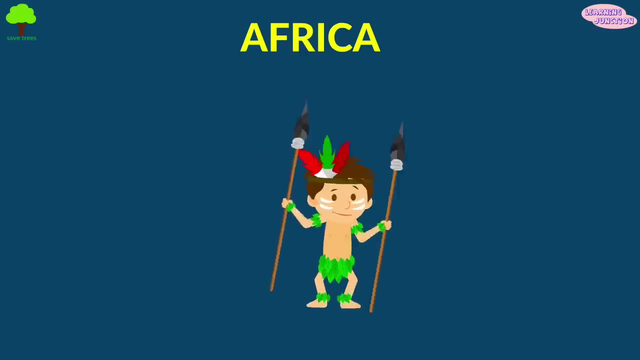 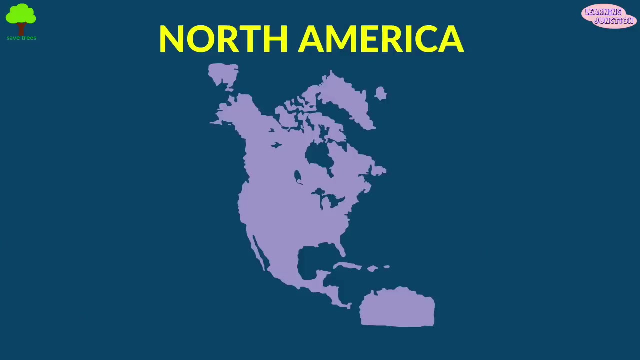 the largest country in africa is algeria. the longest river in the world is the nile in africa, the sahara in northern africa is the largest hot desert- very hot. the most popular attractions are victoria falls in the north, zambia and mauritius, north america. north america is the third largest continent and has 23 countries. 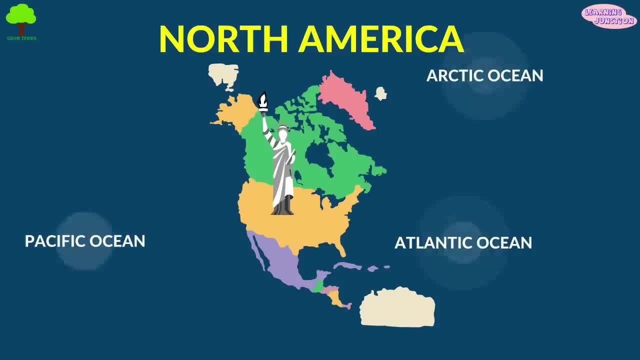 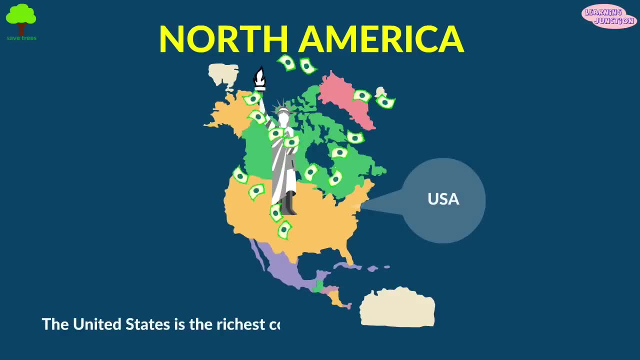 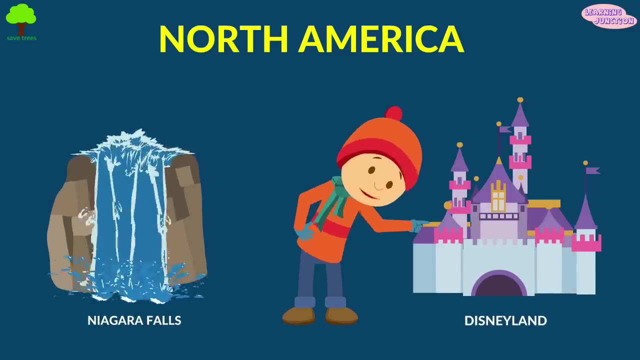 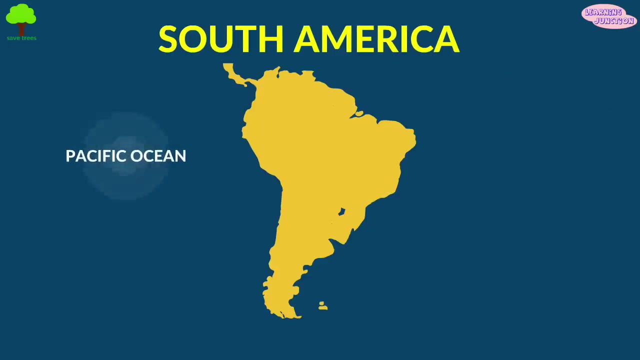 pacific, atlantic and arctic ocean surround it. mexico has the largest population here and the united states is the richest country. popular attractions are niagara falls, canada and walt disney world. united states- south america. the pacific ocean borders south america to the west. 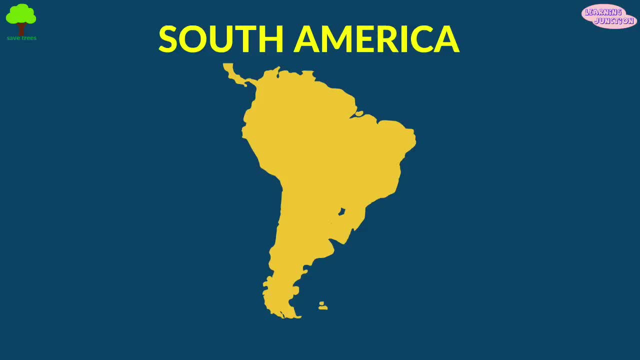 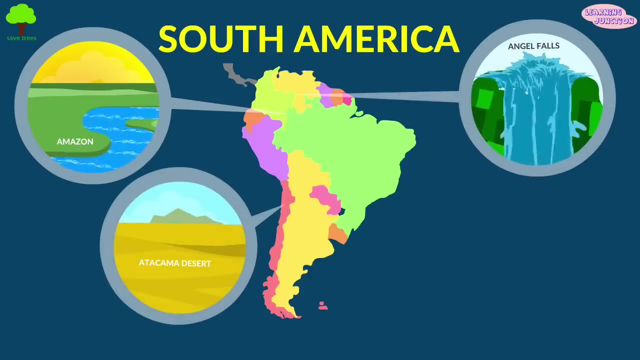 and the atlantic ocean borders it to the east with 12 countries. south america is home to the largest river by volume, the amazon, the world's highest waterfall, angel falls, the driest place on earth, atacama desert and the world's largest rainforest amazon river basin. 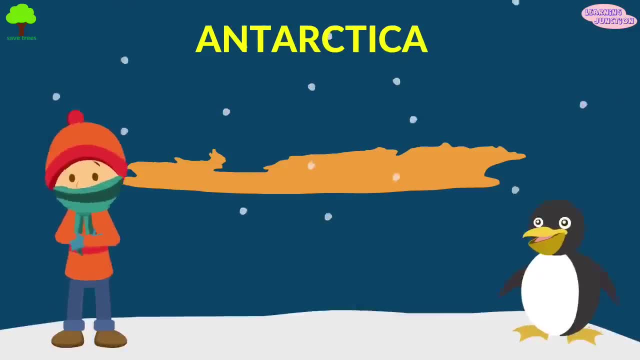 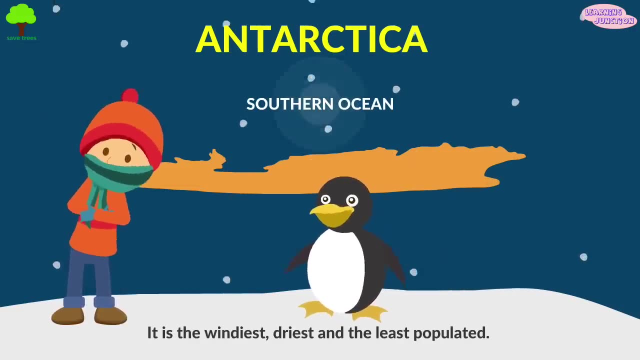 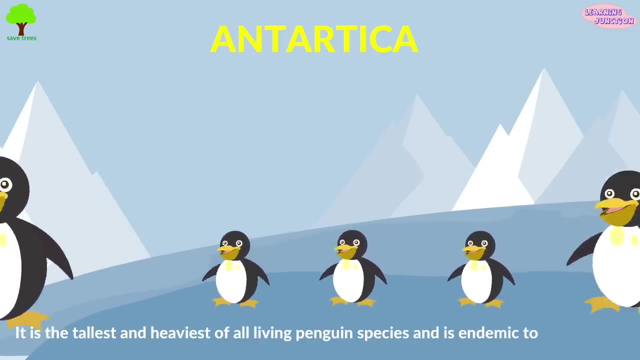 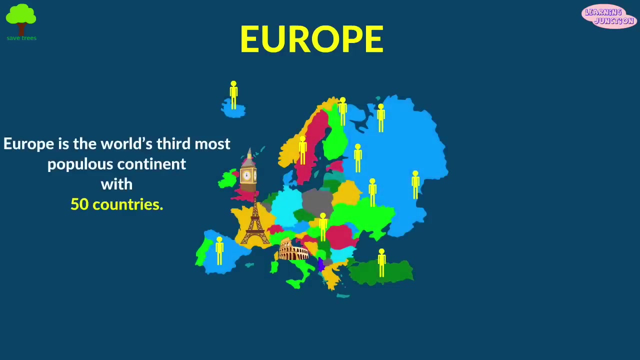 antarctica. antarctica is an ice-covered continent surrounded by the southern ocean. it is the windiest, driest and the least populated. there are no permanent residents on this island. beautiful emperor penguins are found here. europe. europe is the world's third most populous continent, with 50 countries. russia is the largest among these and the 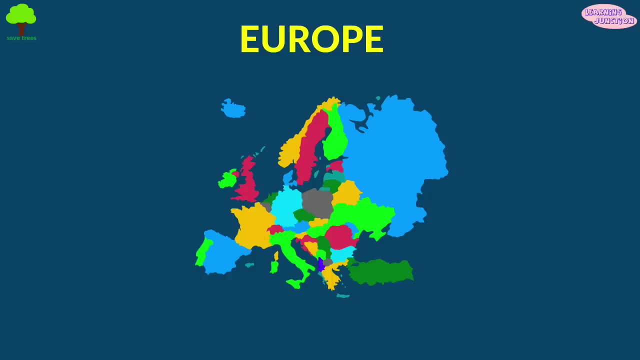 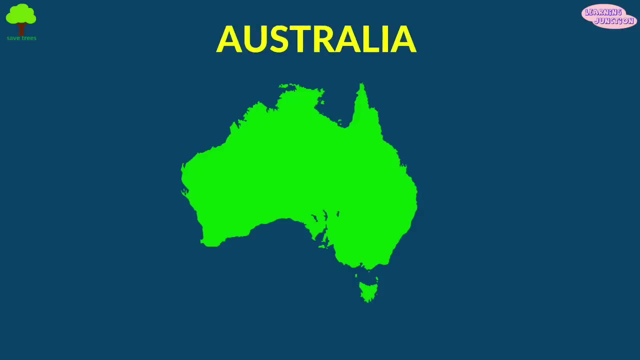 most populous country in the world. the most popular attractions are big ben in england and eiffel tower in france- australia, australia, oceania- is the smallest continent. the main cities here are sydney, melbourne, brisbane, darwin and canberra. the most well-known australian animals are kangaroos. 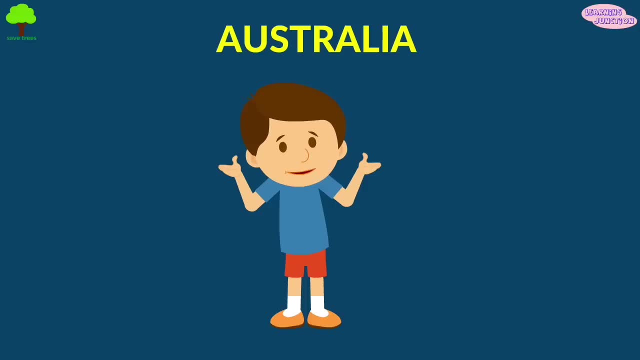 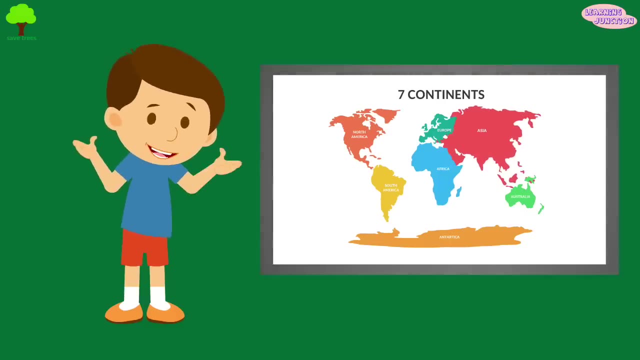 and koalas. the most well-known australian animals are kangaroos and koalas. the most well-known australian animals are kangaroos and koalas. the most popular attractions here are opera house and australian alps. hope you like the video. thanks for watching, bye, bye.